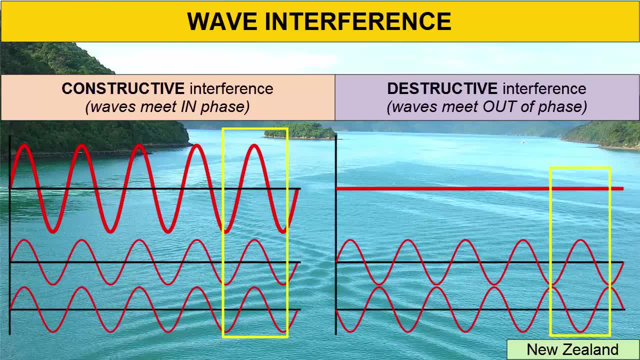 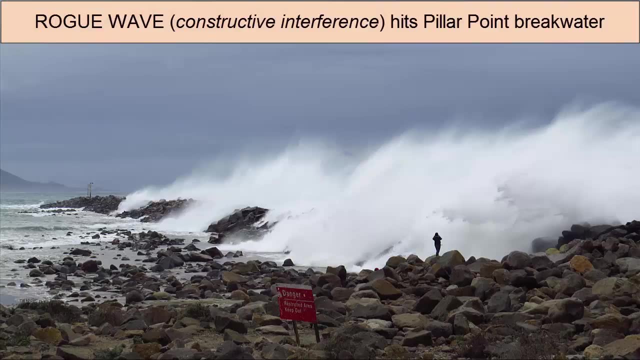 the addition results in a larger wave. When the waves interfere out of phase, the crest of one arriving with the trough of another, they diminish the height of the wave and we call this destructive interference. Ironically, it's the constructive interference that causes the most damage When many large waves constructively interfere in the same. 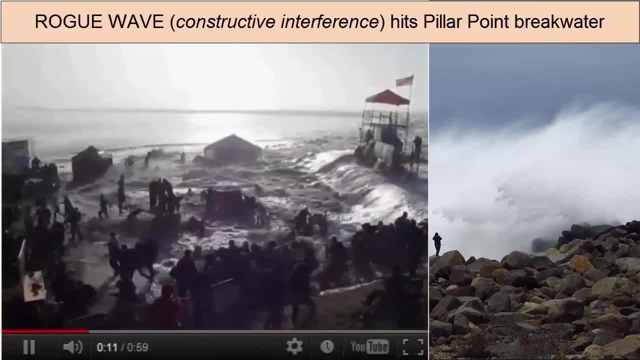 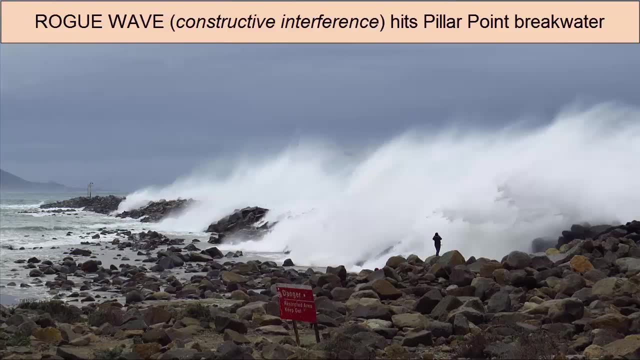 location, they can create a really deep wave, known as a rogue or episodic wave. These are the waves Hollywood likes to immortalize in their movies, where you see a giant waule of water approaching a ravaged boat or coastline. It is also the type of wave that causes the 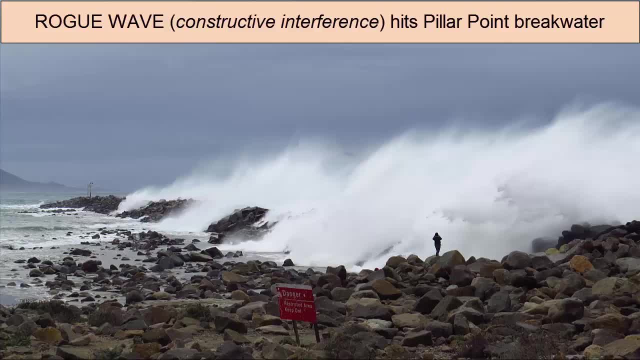 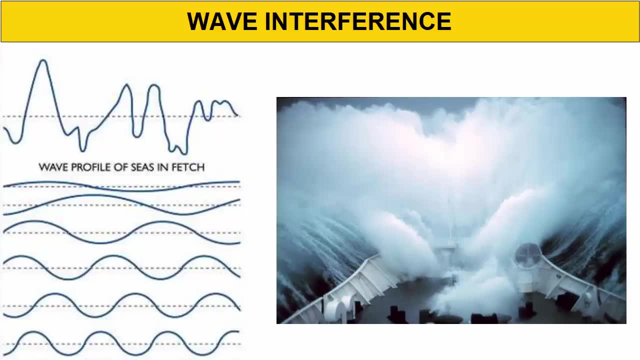 most damage because it has the potential to be the largest. This image shows the waves that result in an area when six different wave trains approach from six different areas. You can see the result of combined interference is a chaotic jumble of waves of varying sizes. 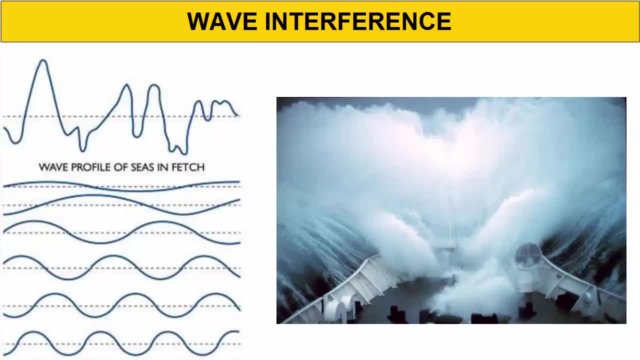 with little consistency. Here you have the makings of a perfect storm where giant rogue waves can develop and shipwrecks are common. How are so many different wave trains created? Some come from different storm systems, but others come from waves from the same storm. 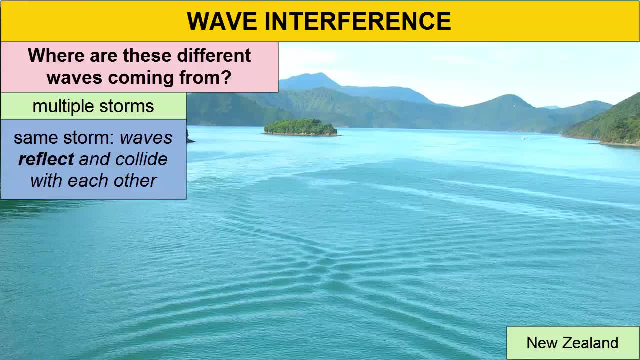 system, colliding with land and reflecting back in a new direction, or having their wave base collide with the seafloor and then refracting or bending around the underwater banks and changing direction. This image of the Georges Banks off of Cape Cod, Massachusetts, a very popular and productive 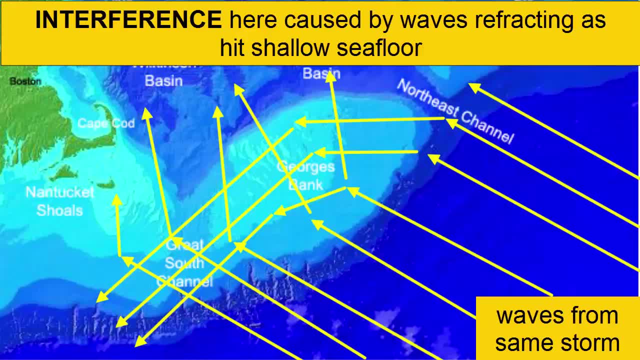 fishing area shows this type of refraction. Waves advancing toward the Georges Bank will slow down when they feel bottom. This can cause the waves to bend almost nonstop. If the waves are in the direction of the seafloor and the seafloor is in the direction of the 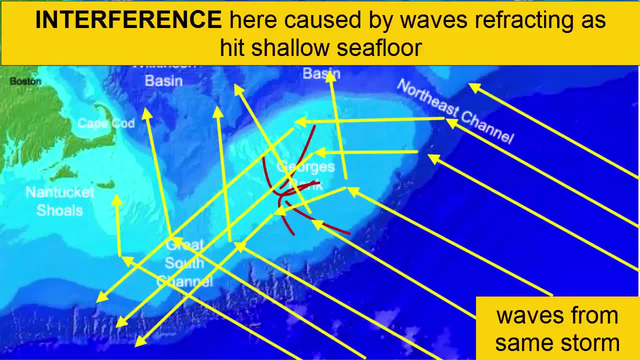 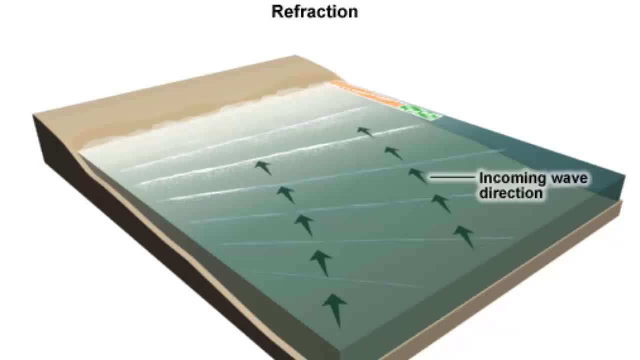 seafloor, the waves will slow down Interference results and the water in this area can be quite erratic and challenging to navigate. You can see this type of refraction when waves collide with beaches. The side of the wave front that feels bottom first will slow down. 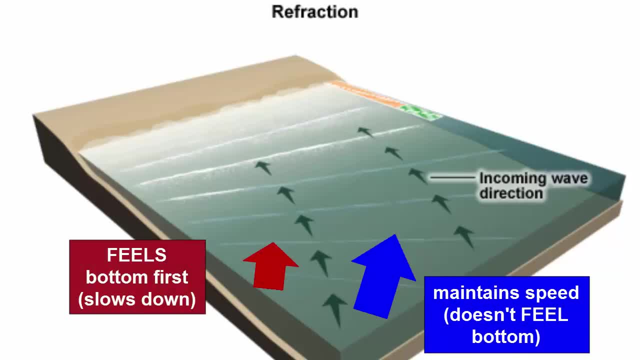 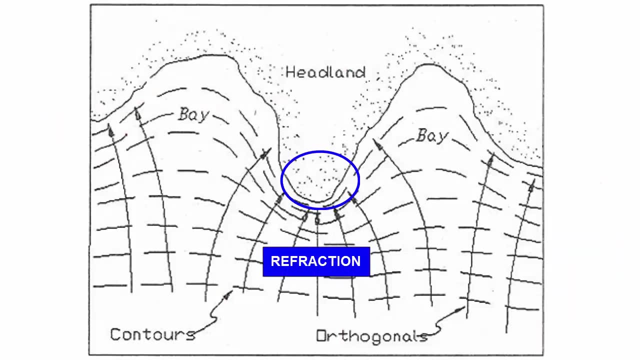 The side in deeper water keeps its speed forward, The net result is a bending inward toward the beach. You see this spectacularly on coastlines that have rocky peninsulas. The waves bend in toward anything that sticks out from the coastline, Focusing wave energy on attacking and eroding these areas. 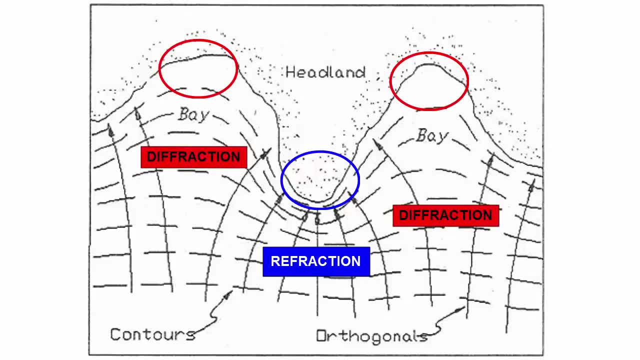 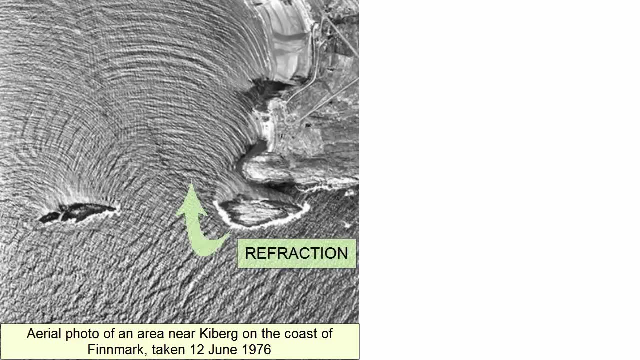 The coves between have waves diffracting outwards, creating much gentler defocused waves inside these areas. So the rocky protrusions have high wave energy, the coves much lower energy waves. This image, taken from above some rocky islands, shows the waves refracting around the rocks. 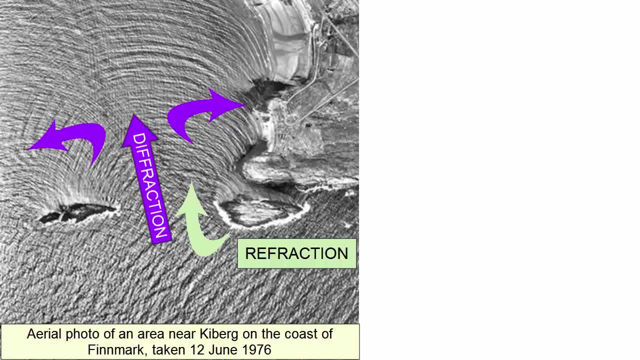 and diffracting through the slot between the two. Another thing waves can do is reflect on the waves. This image shows the waves reflecting around the rocks and diffracting through the slot between the two. Another thing waves can do is reflect on the waves reflecting around the rocks and diffracting through the slot between the two. 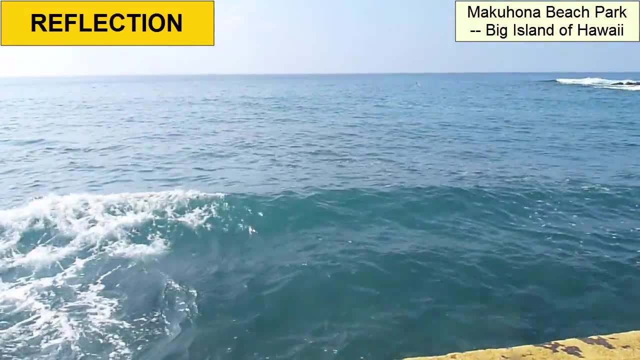 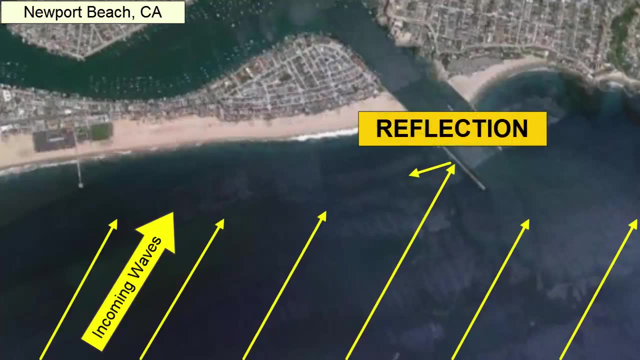 This is especially true where there are hard rocks underwater or human-made walls like jetties. The jetty at the harbor entrance in Newport Beach, California, is well known for its wave reflection. Combined with constructive interference with incoming waves, it creates a large wave called. 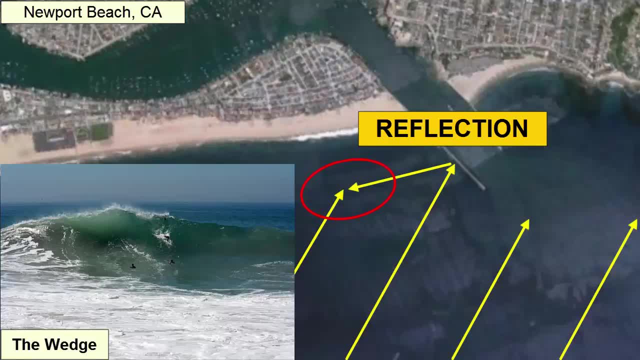 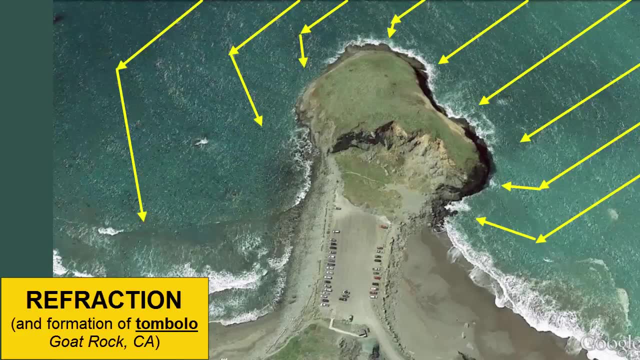 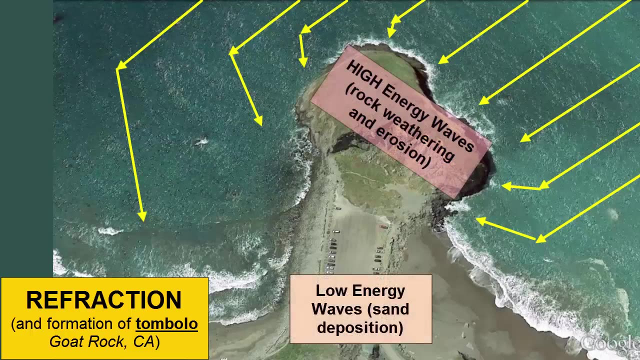 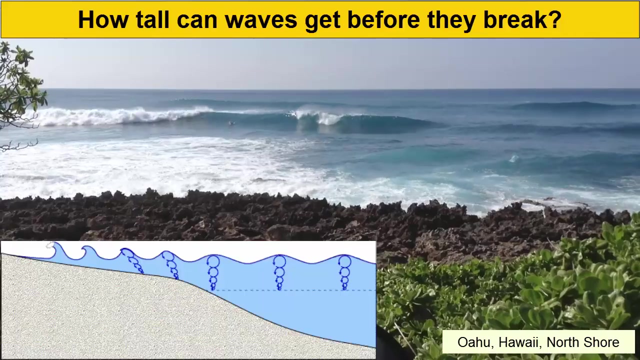 the wedge, which is popular for bodyboarders. This image of a tombolo along the California coastline also demonstrates the refractive power of waves. The waves bend in to attack the rocks that stick out of the coastline and a shadow forms behind it where sand piles up, protected from the high waves that are focused on the island. 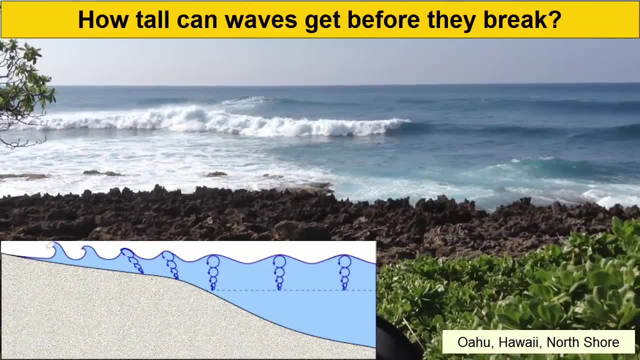 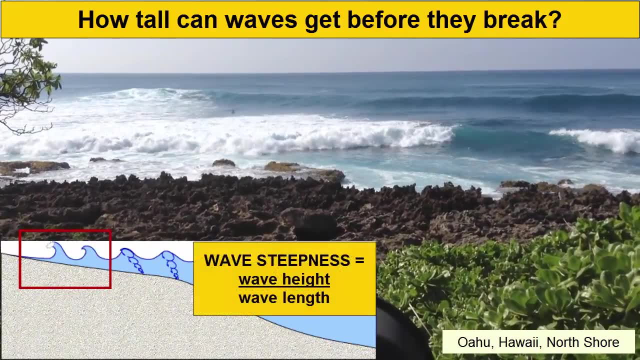 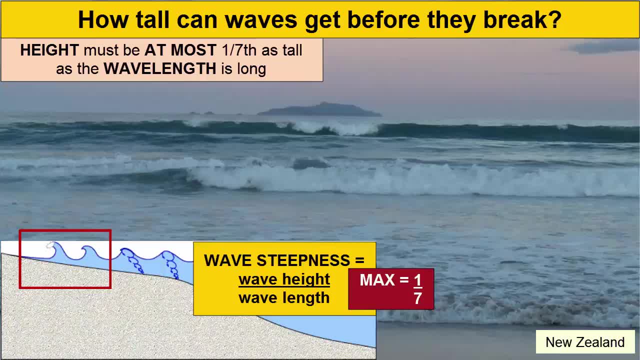 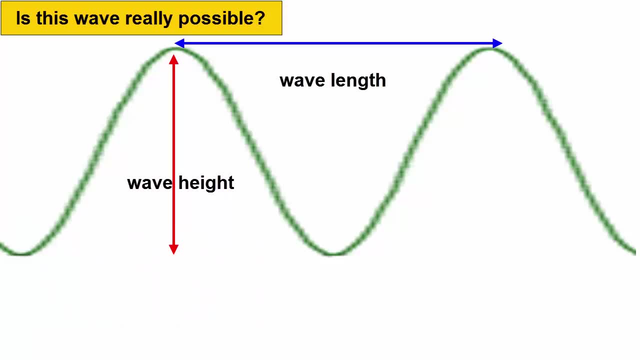 seventh the value of the wavelength, or else the wave will break, Or the wavelength must be at least seven times the value of the wave height. Let's apply that to this idealized wave shape. Is a wave that looks like this really possible? 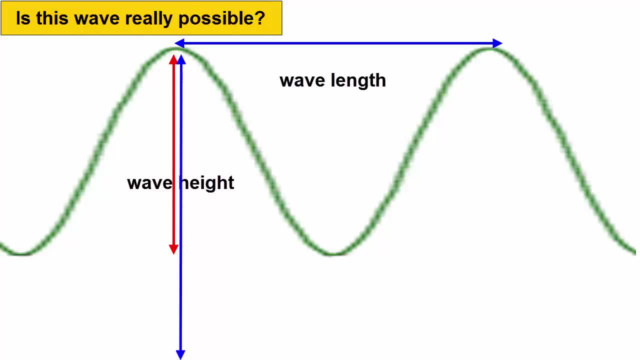 Is its wavelength at least seven times its wave height. Not at all. The wave height is almost equal to the wavelength. at best it's one half the value. It must be shrunk to one seventh before it reflects the maximum steepness a wave can. 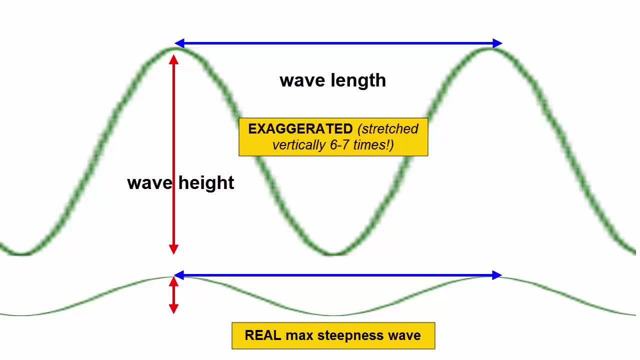 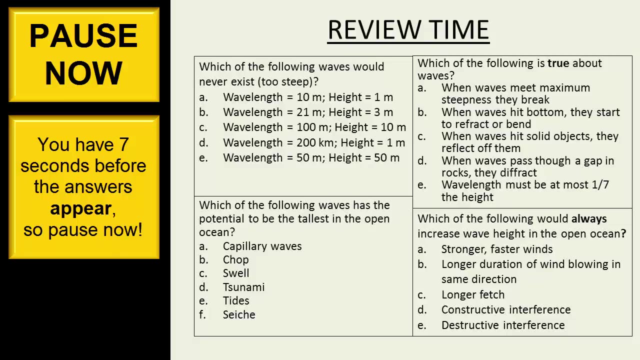 be. Why use the unreal images of waves for teaching? Because it becomes very difficult to show crest trough, height and other characteristics of a wave if it's squashed down to more realistic proportions. Pause now. Most of our conversation so far has been about wind-generated waves, but there's another. 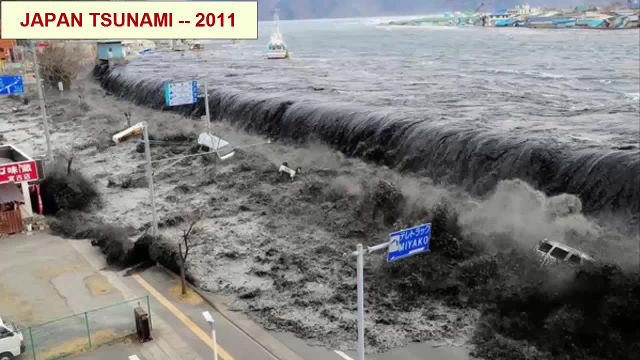 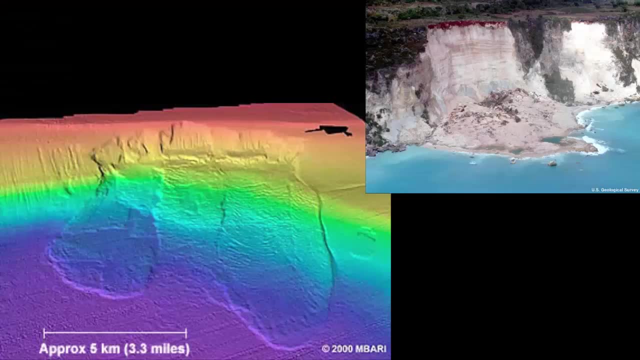 kind of wave we've mentioned a few times: tsunami. These waves are also referred to as splash waves- that result from a large displacement of seawater, either due to a landslide into or under the water, or by vertical displacement of the seafloor during earthquakes. 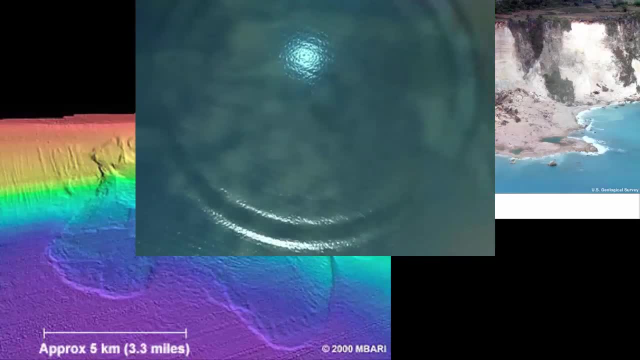 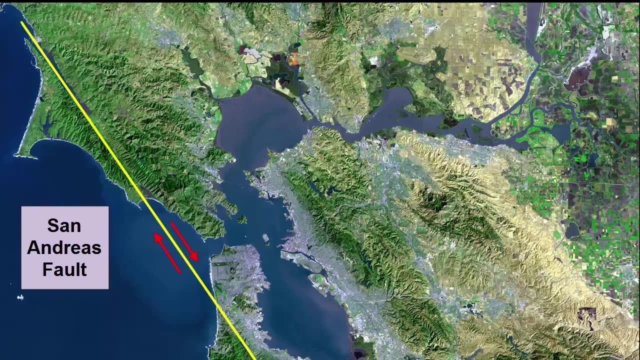 If an earthquake doesn't cause vertical displacement, it will not produce a tsunami. For this reason, the San Andreas Fault, a mostly transformed motion fault, is not associated with producing tsunami, even though parts of it are underwater But seafloor-spreading centers are not. 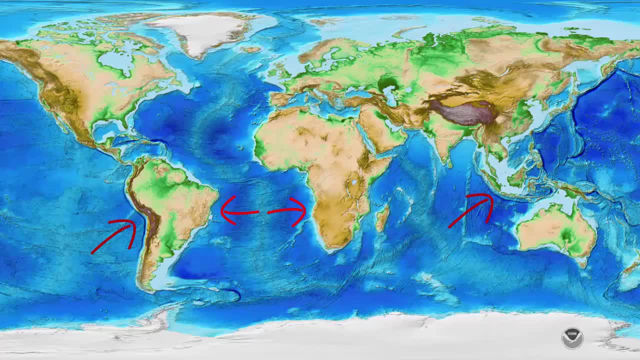 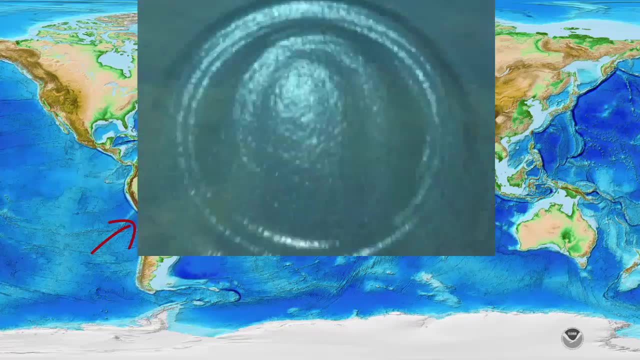 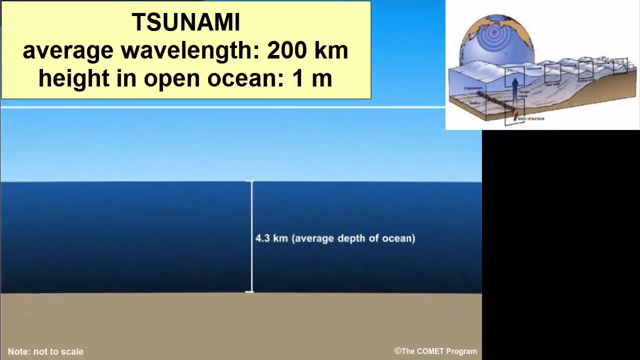 Spreading center earthquakes and subduction zone. earthquakes can produce vertical displacement, and subduction zones are the biggest culprits, as they are associated with the largest displacements. The average wavelength of a tsunami is 200 kilometers. The height in the open ocean is only one meter. 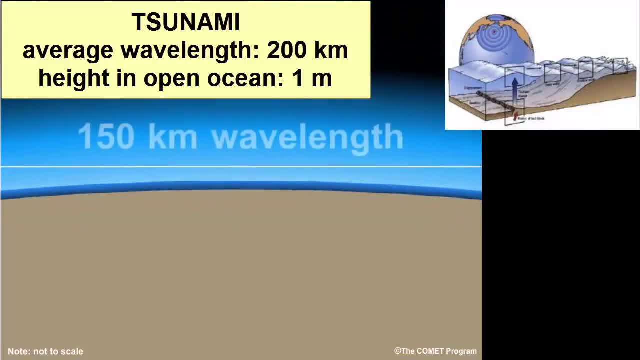 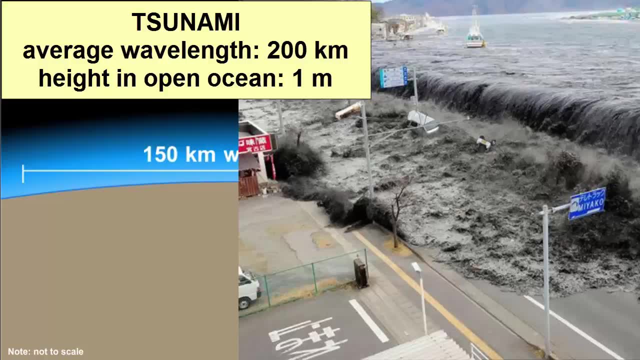 That means the height of the wave should be one two hundred thousandth the wavelength. It wouldn't even appear in this image. It would look totally flat. The height will grow as it approaches the land, as all waves do. The height of the wave should be one two hundred thousandth the wavelength. 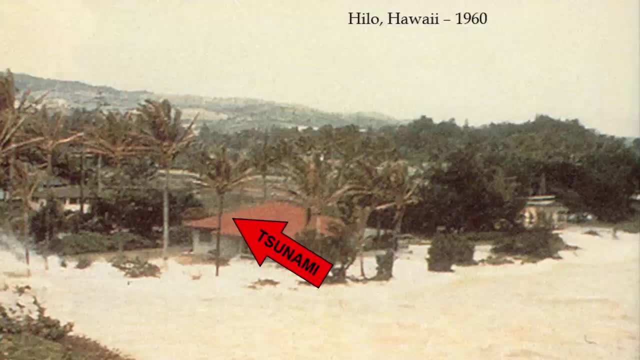 But if the wave reaches a certain altitude, it will still look flat to the observer. This image of a tsunami in Hilo, Hawaii, shows the rising water as an advancing large mass that extends as far as the horizon. It's more like watching a bathtub fill up in front of you, but much faster than expected. 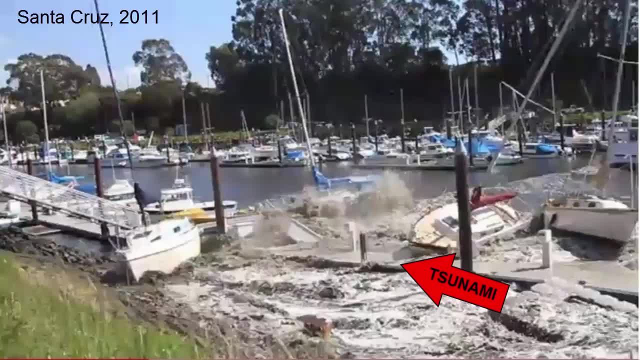 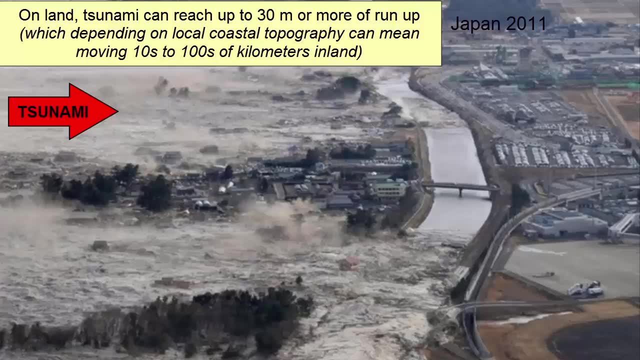 In fact, tsunamis look a lot like the rise and fall of the tides, only instead of the rising and falling happening over twelve hours, it happens within fifteen minutes. Vertical heights of these waves on land can be anywhere from one to ten kilometers. 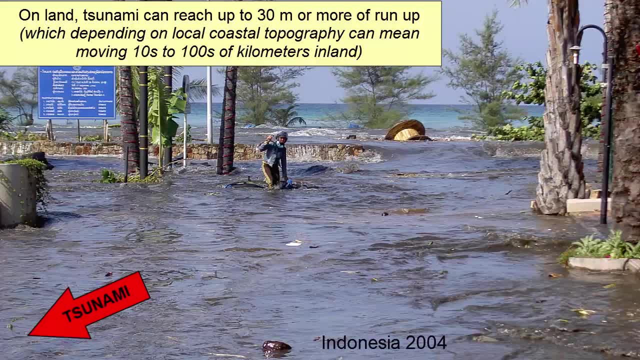 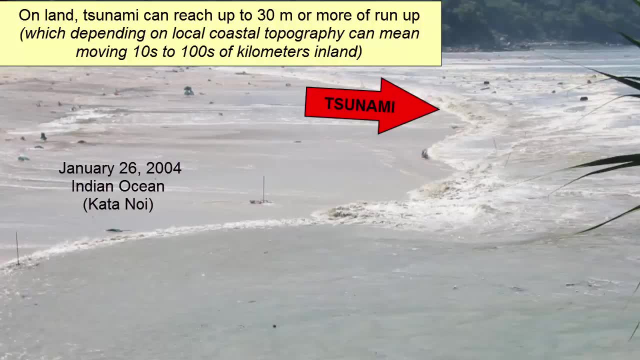 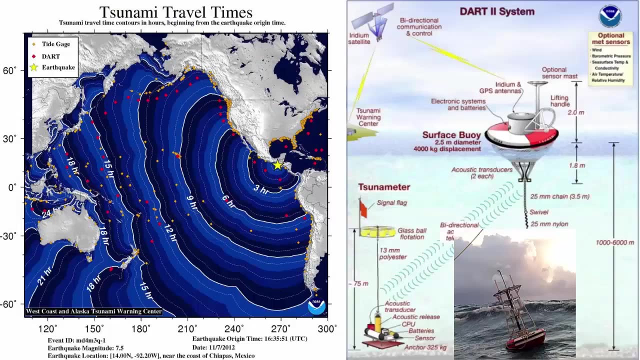 from 1 to 30 meters. For flat land that doesn't have a lot of vertical relief. that means the ocean can penetrate many tens to hundreds of kilometers inland, alternately flooding and exposing the land in cyclic pulses of fast-moving currents of water. The Pacific Ocean, with all its subduction zones, experiences a 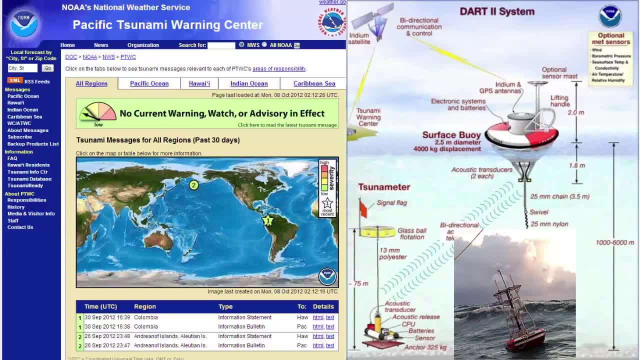 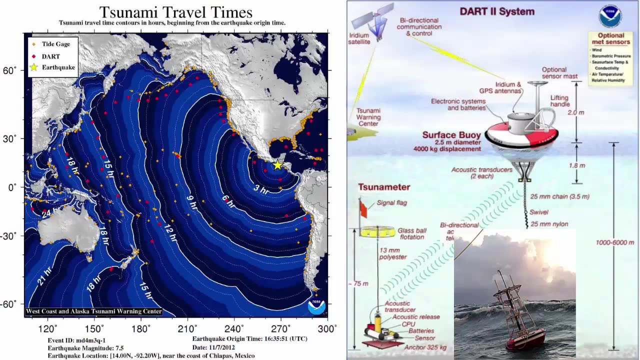 number of tsunami every decade. There is a robust warning system in place to monitor earthquake activity and warn local residents to stay off the beaches. However, not every earthquake will produce a tsunami and not every shoreline will be affected the same way. It depends very much where the tsunami. 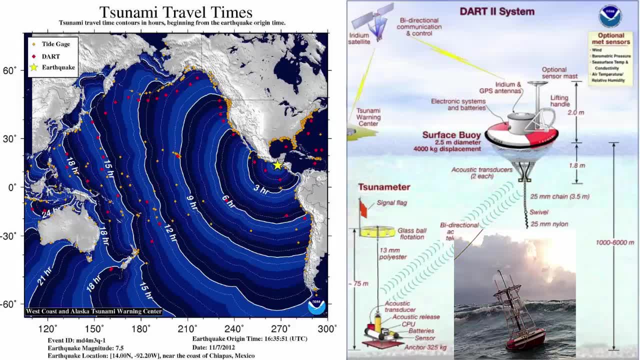 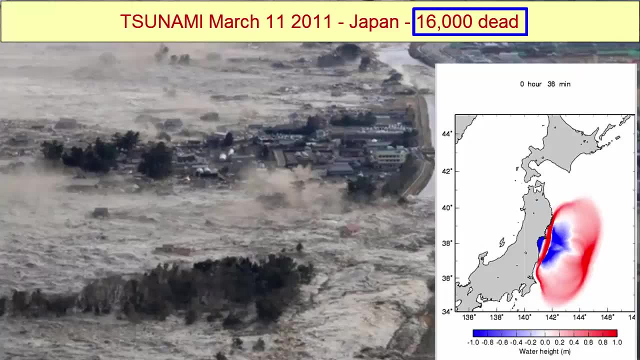 happened and the geometry of the continental slope and shelf off a particular section of coast. For example, the tsunami that hit Japan in 2011 caused significant damage in Japan and its surrounding islands. The wave arrived at beaches throughout the Pacific Ocean and reached different heights in different 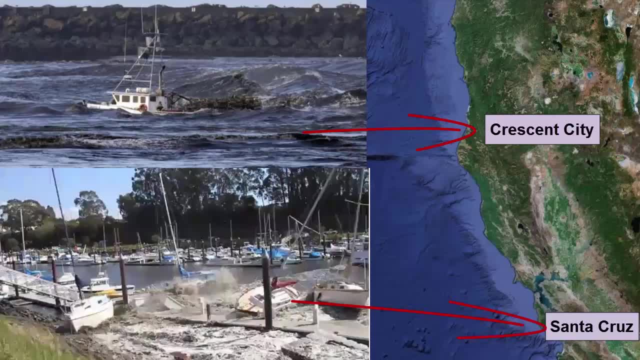 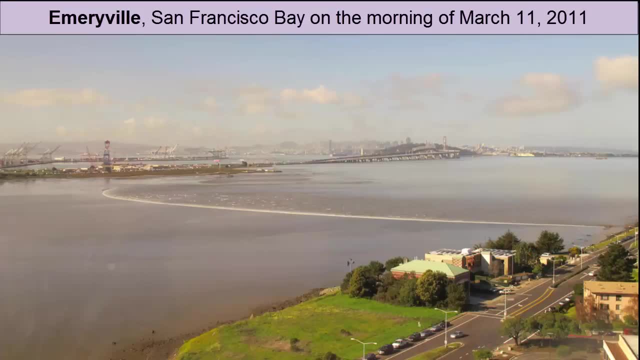 locations In California. there was damage in harbors in Crescent City and Santa Cruz. Remember it was the energy that transferred across the ocean as waves, not the water. In fact, it takes one to two years for the debris produced by that tsunami to wash up onto the beaches. 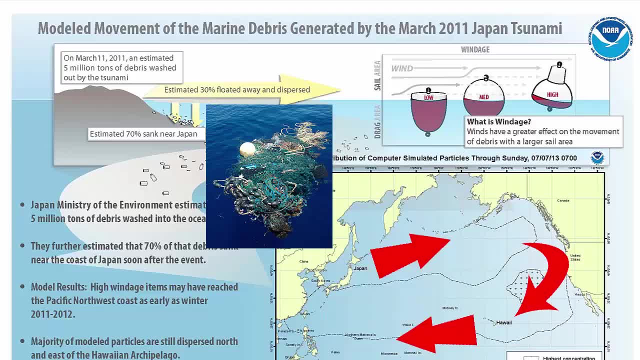 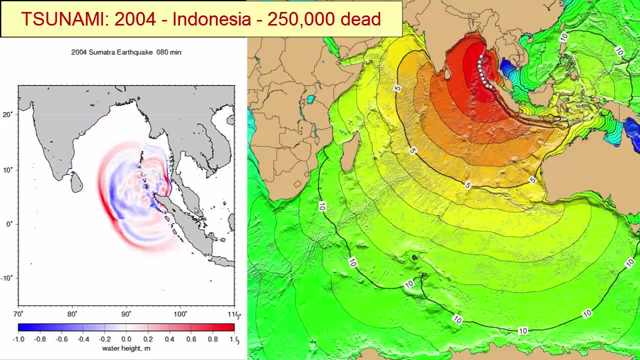 of North America carried by ocean currents. In the 2004 tsunami in the Indian Ocean, there was no way to warn the residents of the impending tsunami because there were no warning systems in place on the beaches. The Pacific Tsunami Warning Center had an alert to provide, but there was no way to transmit that information to those. 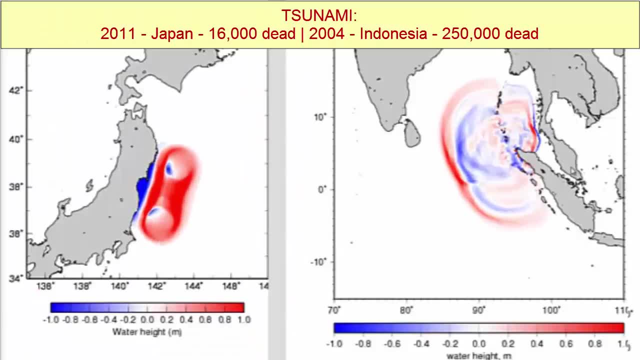 who would be affected. These two images show the propagation of tsunami waves outward from the Japan 2011 earthquake and the Sumatra 2004 earthquake. You can see the effects of refraction, as well as the fact that sometimes the crust of the 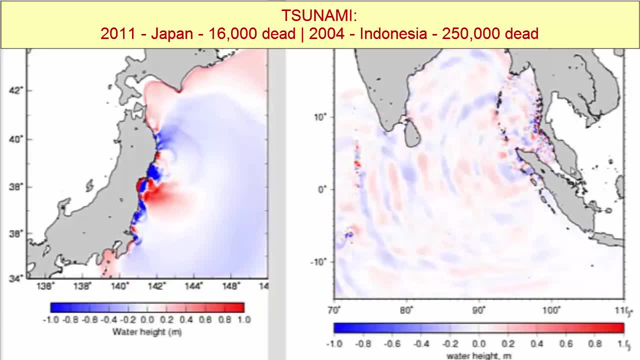 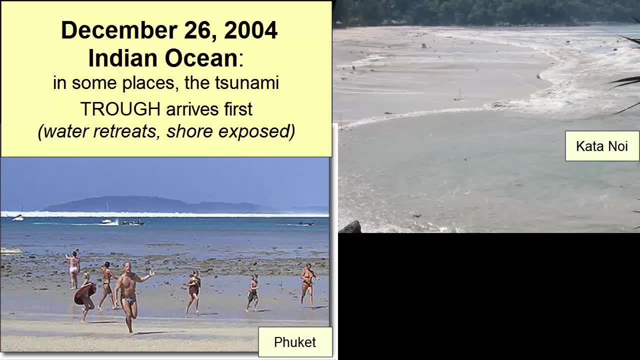 tsunami arrives first- red, and sometimes the trough arrives first- blue. When the trough arrives first, folks see water removed from the beach and often that causes people to move away from the beach. When the trough arrives first, folks see water removed from the beach and often that causes people to move. 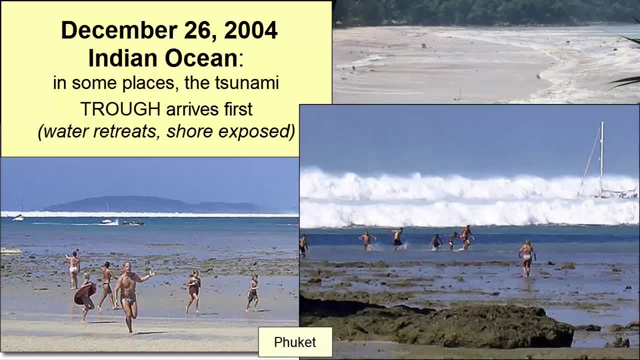 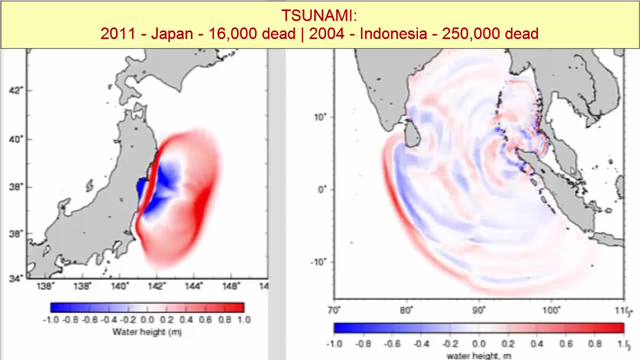 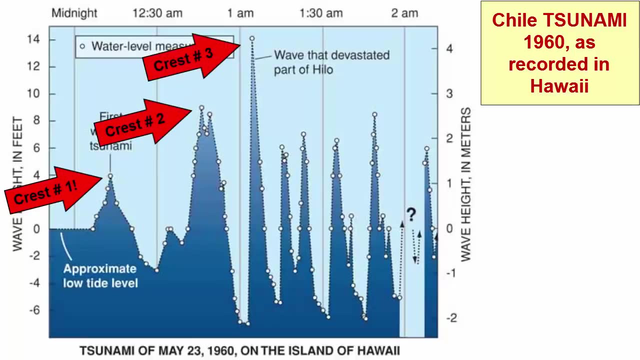 about into the inner tidal area to explore. They then get caught in the crest when it arrives. Typically, there are about four to eight individual waves in a tsunami train. Height can vary throughout. Often it's the second or third wave to hit that has the highest amplitude. 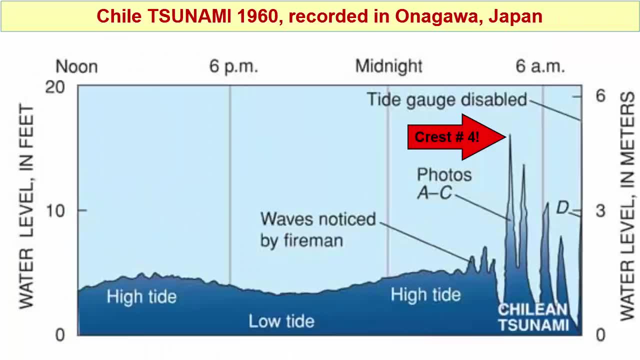 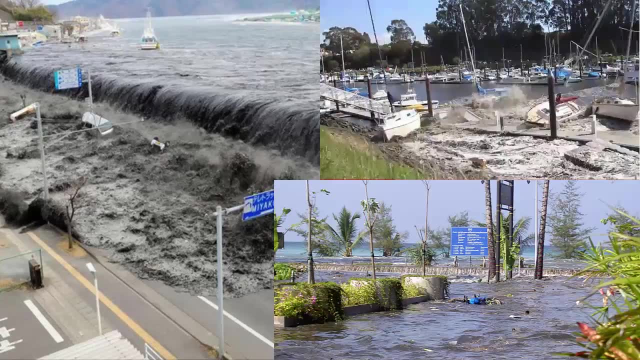 Education on tsunamis lasts only as long as local memory of the last one. If you plan to travel to or live in an area prone to tsunami, it's good to pay attention to signs from the ocean and know your escape route. If you see water rising or falling, quickly head to high ground right.